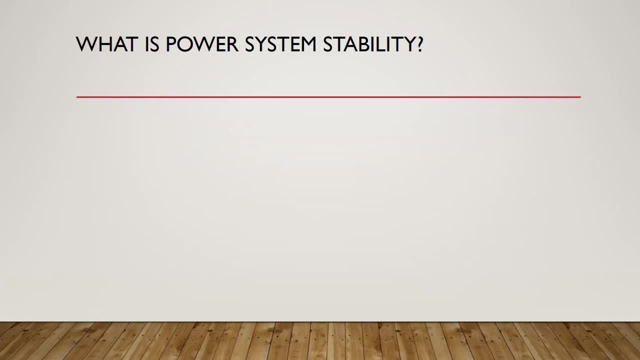 So, first, what is the power system stability? It is the ability of an electrical power system, for a given initial operating condition, to regain a state of operating equilibrium after being subjected to physical disturbance, so that the system or the entire system remains intact. So what does it mean? It means that our power system, or the power system stability. 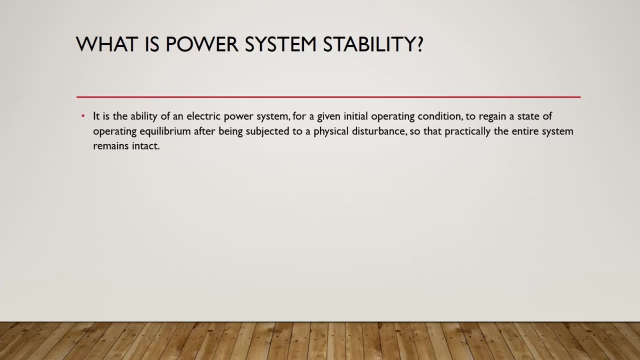 We are saying that the power system is stable When the power system is able to to gain a state of equilibrium. if the power system can have a steady state, for example, if we are talking about the frequency, the power system reaches a steady state frequency. or if we are talking about voltage, it reaches a steady state, or a constant value of a voltage maintained at all bosses. 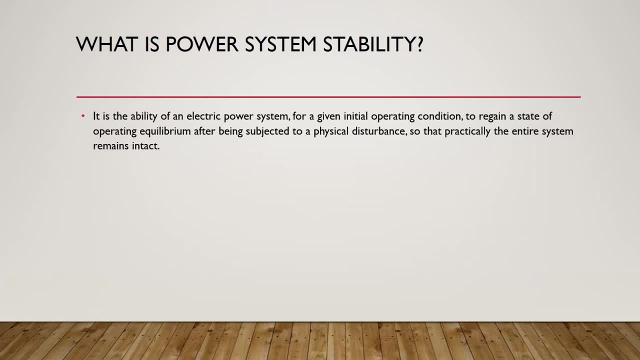 This is an example. This is an example of the meaning of an operating equilibrium state. Physical disturbance means that our power system is subjected to disturbances such as the variation in the mechanical input power to our generator or a change in our load: an increase in load or a decrease in load. 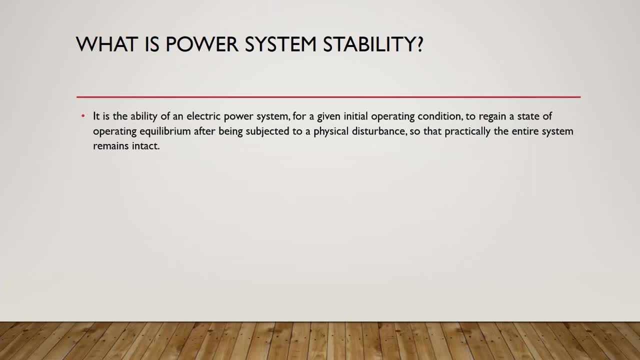 This is considered as a physical disturbance to our power system, which is a fault on transmission lines. this type is also considered to be a disturbance. so let's see if our system is stable or not stable after being subjected to these different types of physical disturbances. so this is the definition of power system stability. the 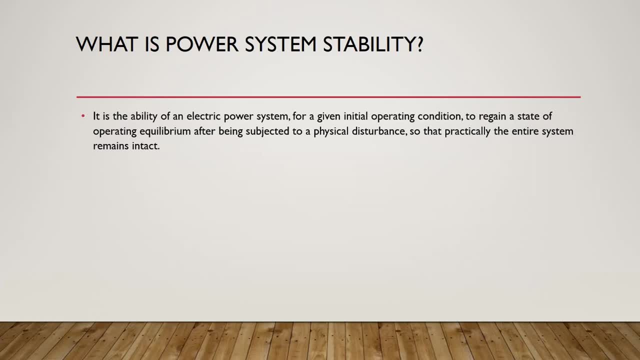 electrical power system is, or having the ability to be, in a steady state condition or an equilibrium state after being subjected to these different types of disturbances. so this definition is applied to an interconnected power system as a whole, for example, a group or a large group of generators connected together. 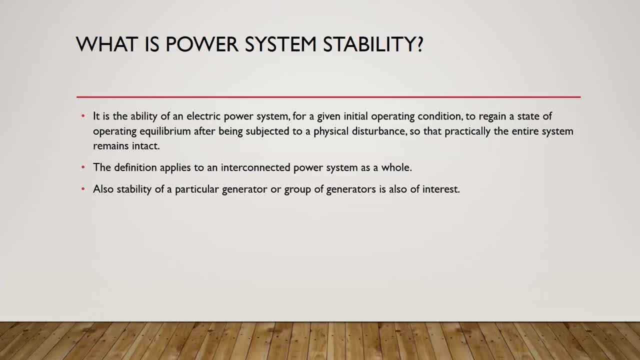 and also can be for one particular generator. as an example, if a generator loses its stability or the meaning of stability here, the synchronism- it is now not synchronized with our power grid and will under identify what is the meaning of synchronism in the next slide. so the generator may lose synchronism, but our system is still stable. okay, the generator. 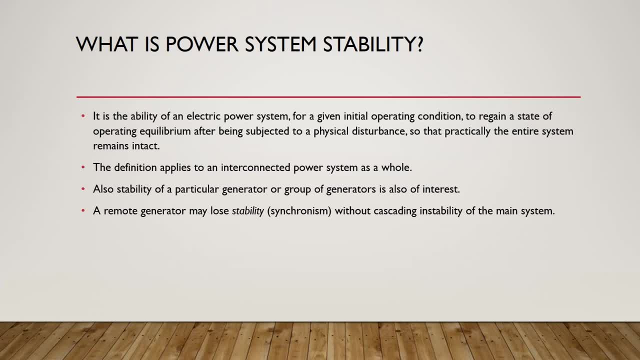 itself loses its stability. so when we are talking about this, we are talking about the stability of the one particular generator, not the stability of our power system. or we can say also the stability of group of loads or a load area, for example. the motors itself can lose a stability, for example, the motor, as you know that as an example, 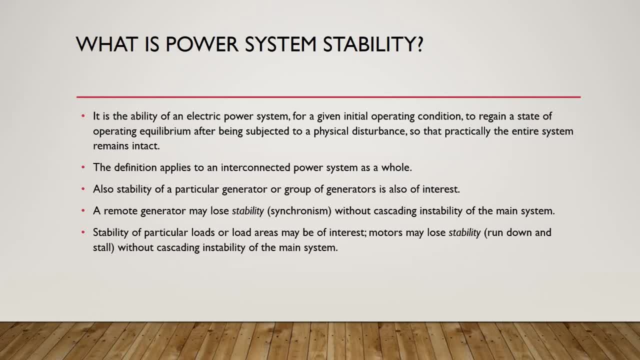 the induction motor. the torque in the induction motor depends mainly on the voltage. So if we have a voltage instability- the voltage, for example, decreases below a certain value- then our motor will need to absorb a lot of current or withdraw a lot of current in order to produce the same torque for the loads. 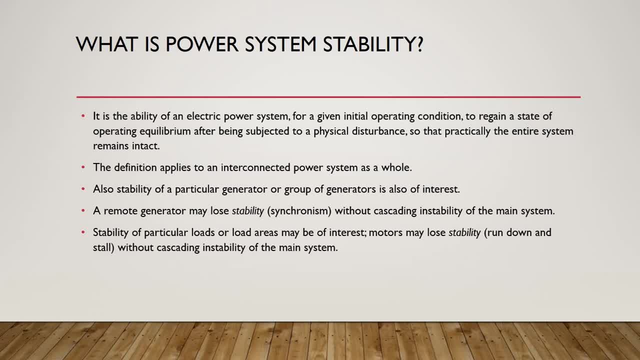 So the motor itself will be overheated by the presence of large current in order to produce the same torque. So the protection devices will turn off our motor or disconnect our motor. So this one means we are talking about the stability of our motor. The power system is still stable, but our motor is unstable. 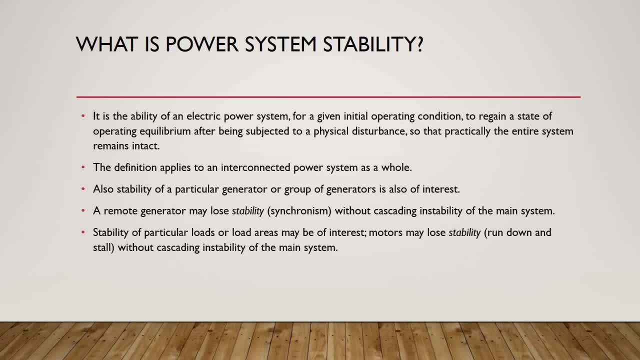 So we can talk here about the Stability, about the group of connected or interconnected power system or a generator or a group of generators, Or we can talk about one generator or stability of a group of loads or particular loads or an area. The stability of the system itself depends on the initial operating condition and the initial operating of our generator. 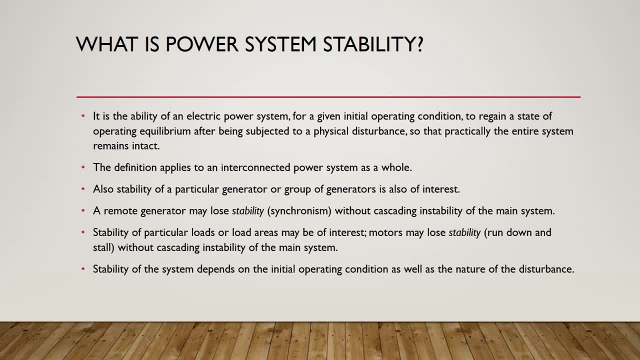 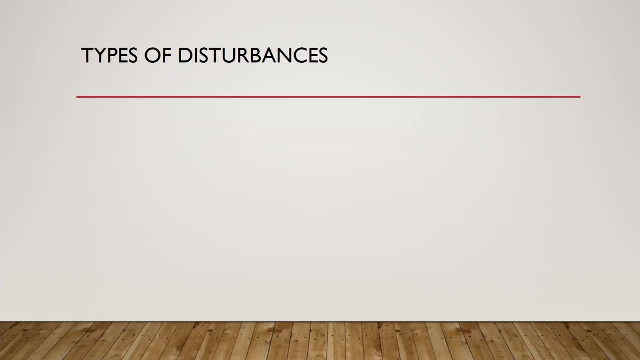 For example, And the type or the nature of our disturbance, The types of disturbances that our power system can be suffered from, The small disturbances, a small change in our power system. This can be in the form of load changes, which occurs continuously in our power system. 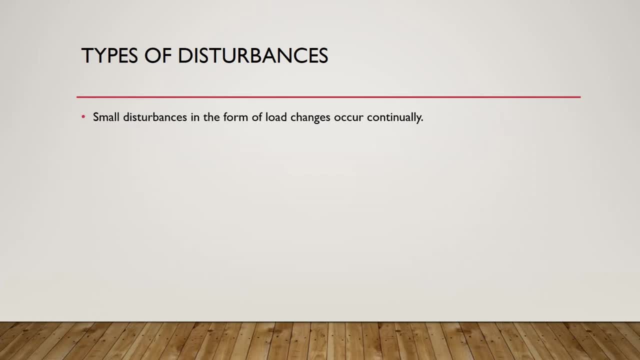 The variation in load. the load can increase or decrease, As you know that our load In our power system is not constant, So our load can increase or decrease continuously through the time. A large disturbance in our power system, such as a short circuit on a transmission line or a fault on transmission line, 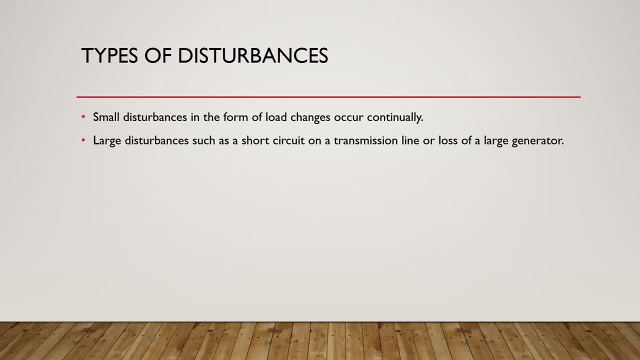 Or the loss of a large generator which can cause imbalance or unbalance between the generation and the load, This is considered to be A large disturbance. The system must be able to adjust to these changing conditions And operate satisfactorily In case of having a small disturbance or large disturbance. 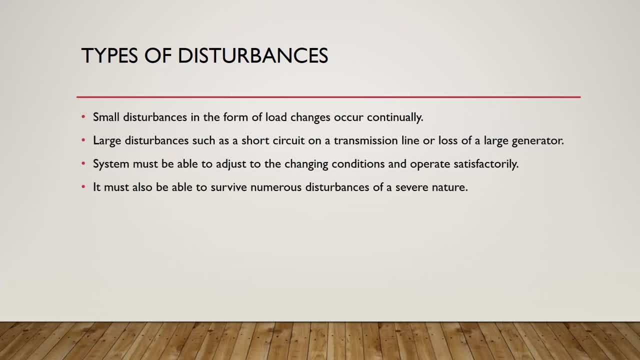 So it must be able to survive this numerous amount of disturbances of the severe nature. So our disturbances, such as the large disturbance, Such as the large and small, The power system should be able to adapt to these different disturbances. Of course, we cannot contain all the cases or all the possible large disturbances and small disturbances in our power system. 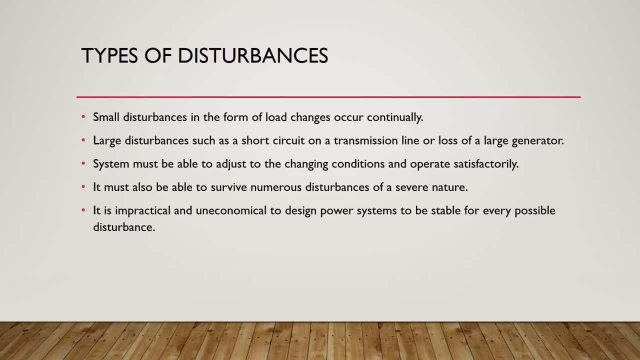 Because it is impractical and uneconomical to design our power system to be stable for every possible disturbance. So what are we going to do? We are going to choose the most or the cases which have the most probability of occurrence. So we don't design our power system for every possible disturbance. 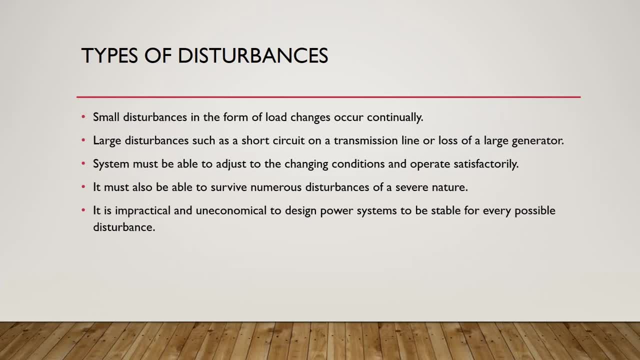 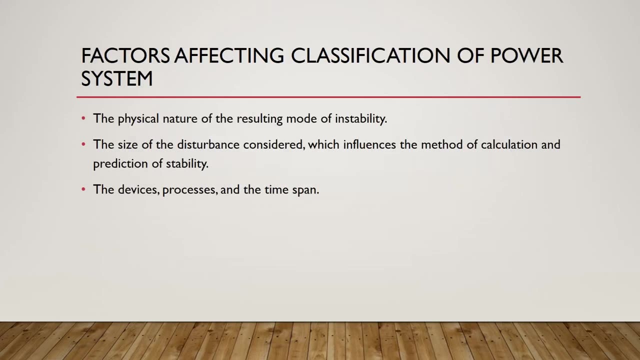 But we design our power system for the most cases or the most disturbances which will happen, Which having the highest probability. So the criteria is based on the high probability of occurrence. The factors affecting the classification of power system stability Number one: the physical nature of the resulting mode of instability. 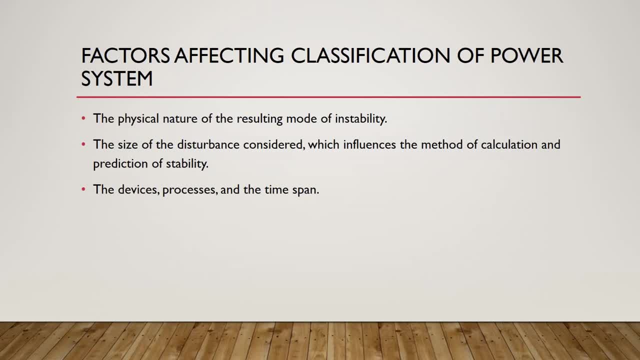 Is it instability in voltage, Instability in frequency, Instability in the rotor angle? Number two: the size of the disturbance. Is it a large disturbance? Is it a small disturbance? In these different cases, we will have a different method of calculations. 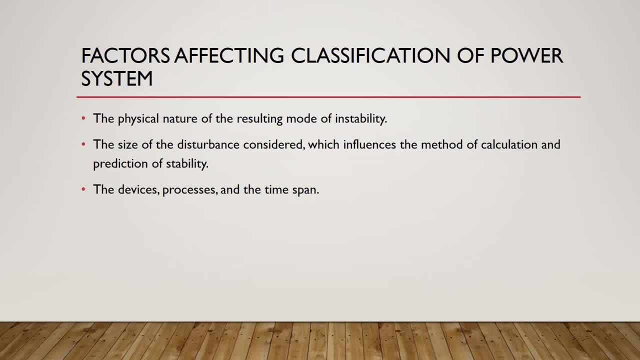 For example, in small disturbances we can linearize our equations, But in the large disturbance it is not practical to linearize the equations. Number three: the time spans, the devices and the processes. In this case we have, for example, 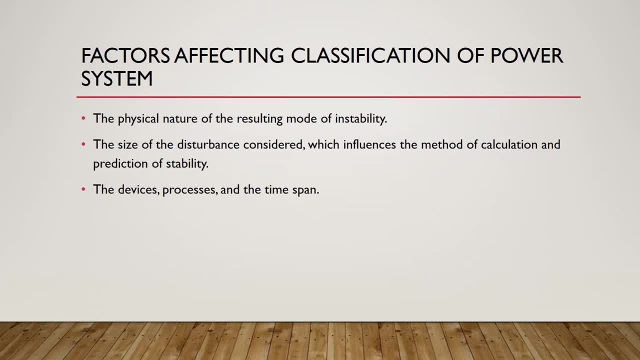 short period, or a short duration and large duration. Some disturbances need to be examined for a large period of time And others for a short period of time, As we will see in the next slides. So first we need to identify the condition of synchronism. 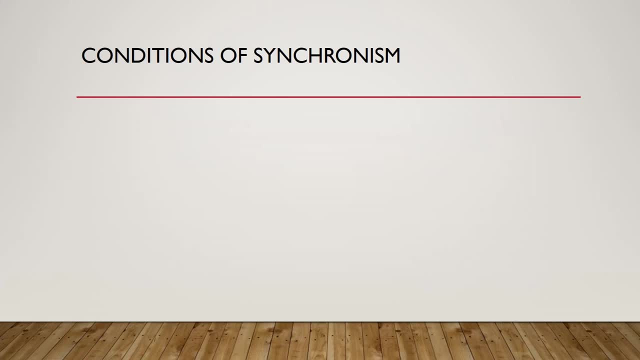 Synchronism. what does it mean? It means that our generators are connected in parallel or connected to our power grid, And these generators should have the following conditions. The first thing: they should have the same voltage, Each of them, the V line to line or the V phase. voltage or V phase. 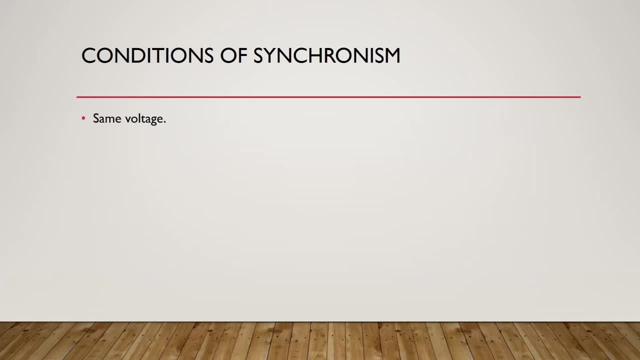 should have been the same in every generator inside our grid. Each generator connected to our grid, The second one. they should have the same frequency. For example, in my own country we use 50 Hertz, Some countries use 60 Hertz. 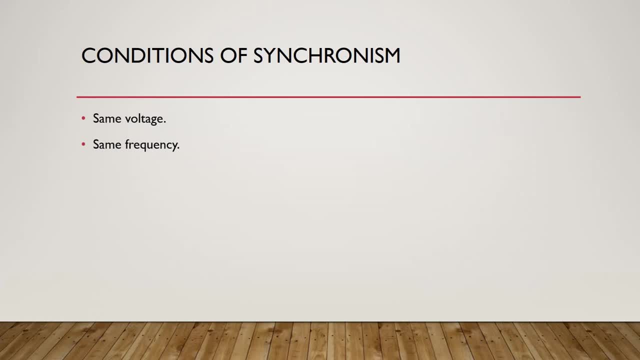 So all of our generators should have the same frequency, They should have the same phase shift or same initial angle. You know that the sine wave or the voltage is sine omega t plus an angle called the phi, which is the phase shift. So the phase shift should be the same in every generator or in every three phase system. 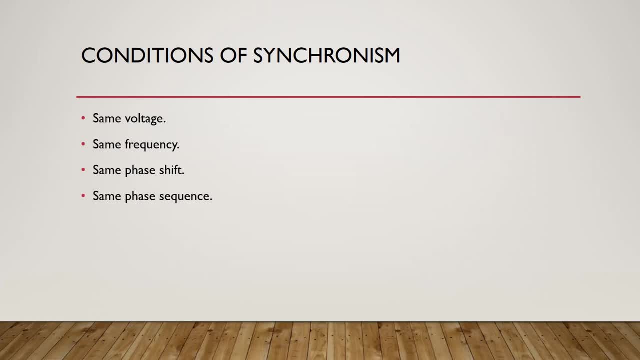 The fourth thing, which is they should have the same phase sequence, For example, as we remember that phase A is sine omega t and phase B is sine omega t minus 120 degrees, And phase C is sine omega t minus 120 degrees. 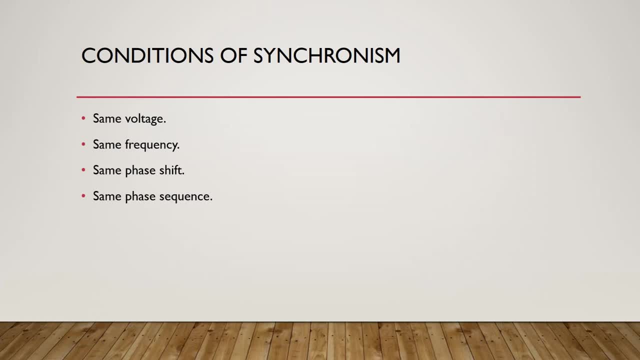 So phase A inside the generator number one is the same as phase A in generator number two, Same as phase B in the generator number one, Same as in generator number two, and so on. So phase A for every generators are connected together And phase B are connected together. 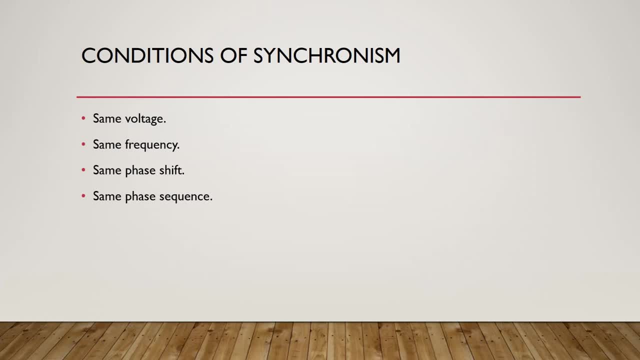 And phase C are connected together. The fifth thing is they should have the same wave force. Every waveform or every generator output voltage should have the same waveform. Everyone should have a sinusoidal waveform, of course, So they should have the same sine wave. 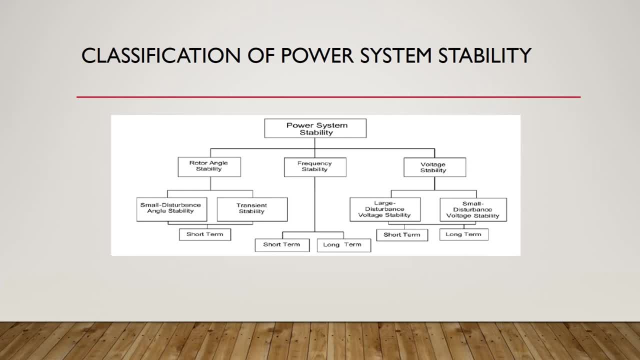 So what are the classification? What is the classification of power system stability? Our power system stability is divided into three main types: The rotor angle stability, The frequency stability And the voltage stability. The rotor angle stability has two types. In case of a small disturbance, 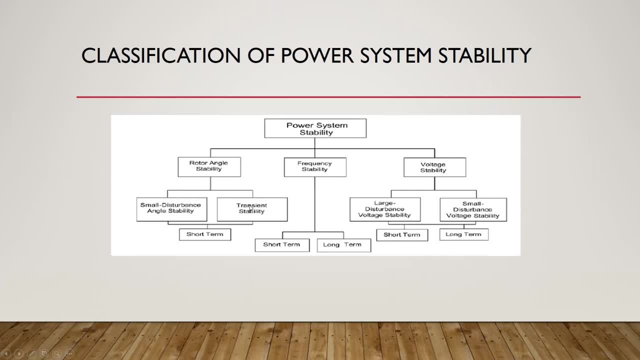 And in case of a transient or large disturbance, And all of them are a short term or for a short period of time. The second type, which is the frequency stability, Which has a short term and long term. The third one, which is the voltage stability. 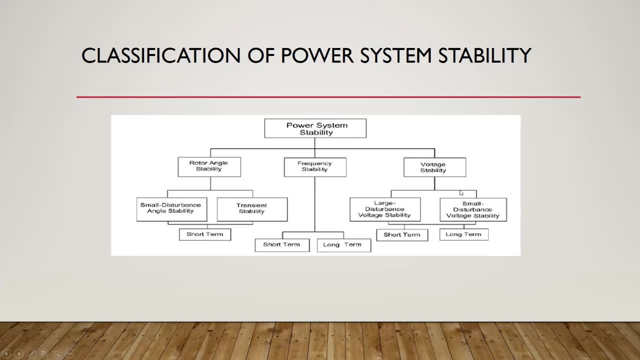 Which is consisting of large disturbance and small disturbance, And also have the voltage, have a short term and long term. In the next video we will start discussing the rotor angle stability And frequency stability And another video for voltage stability.